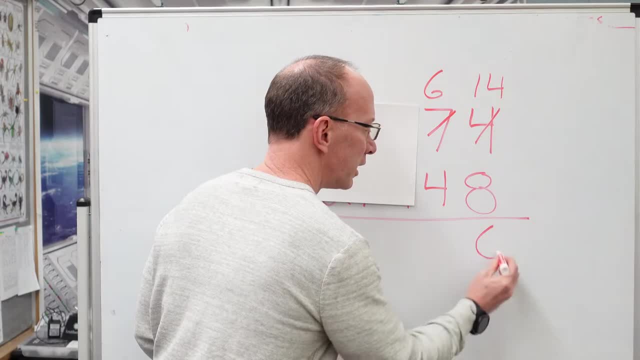 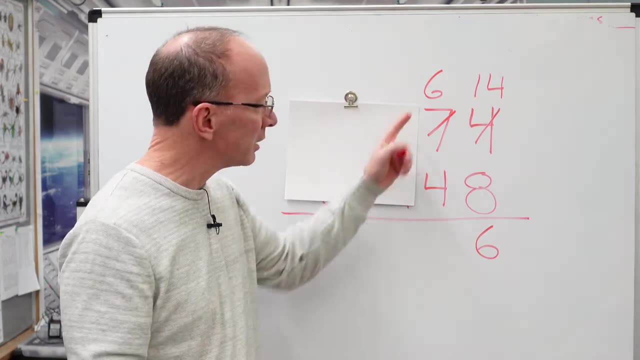 10,, 11,, 12,, 13, 14.. We put a six over here, We start subtracting the tens and now we move it over. Can we do it? Six minus four. I got six cookies. You want four of them? I can do it I. 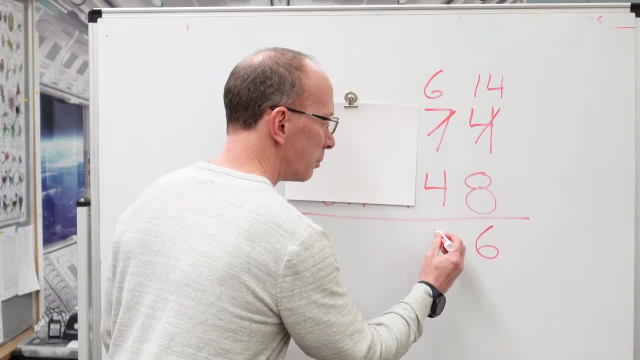 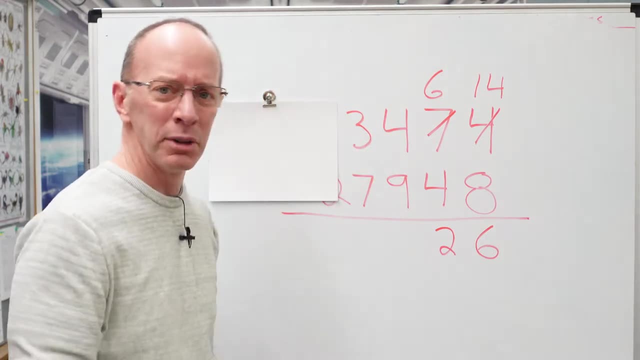 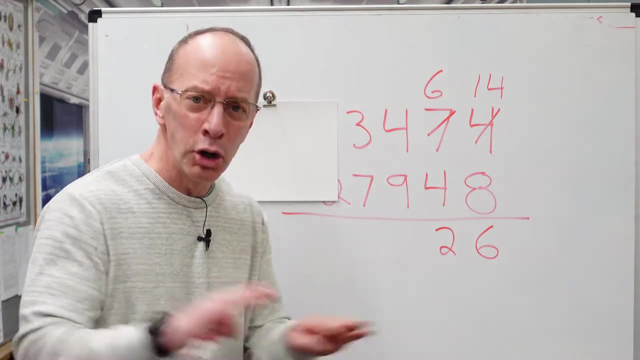 can share some of my cookies with you. So six minus four would be two. I'm going to move this paper over here. I think we can start dealing with some of these other numbers Not too scary right now. Four minus nine Can't do it. This number right here, too small. Need to borrow from our. 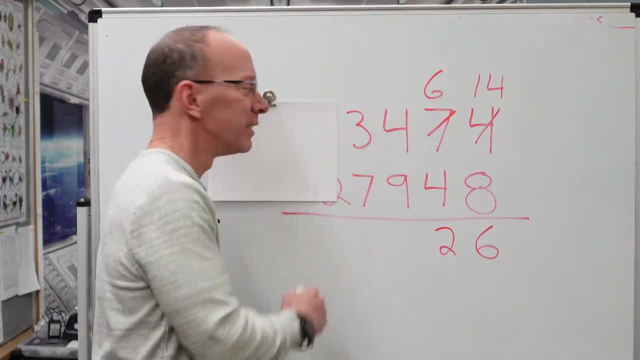 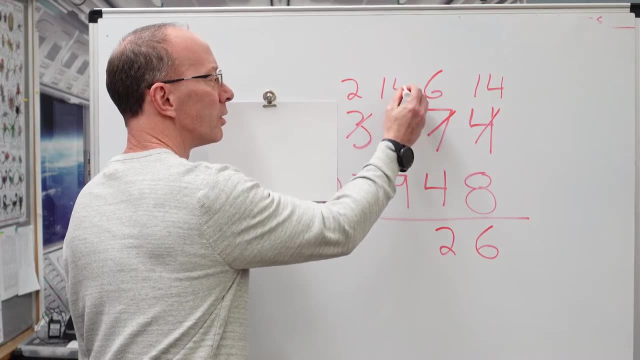 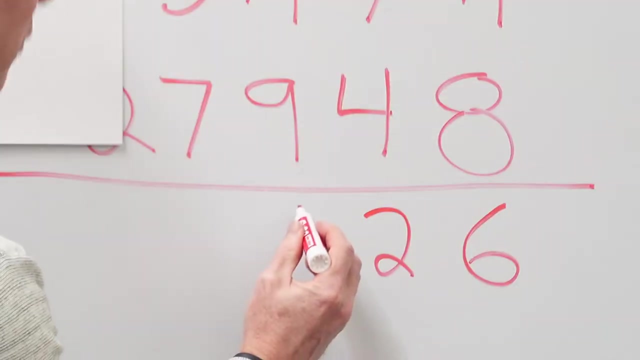 next door neighbor. Hey, can I borrow Some from you? Yeah, So I just borrow one from that. three, Make this a two. Put a line through here. This is a 14.. All right, 14 minus nine, nine, 10,, 11,, 12,, 13,, 14.. So I put a five right. 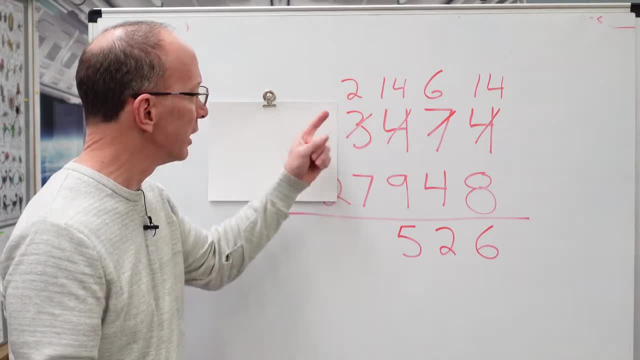 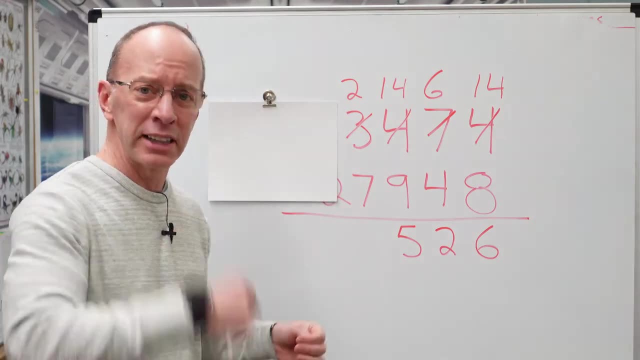 here. Go on to the next problem. Can I do it? I got two. I need to take seven. I can't do it. I got two cookies. You want to take seven, Can't do it. Got to go over to the next door neighbor. 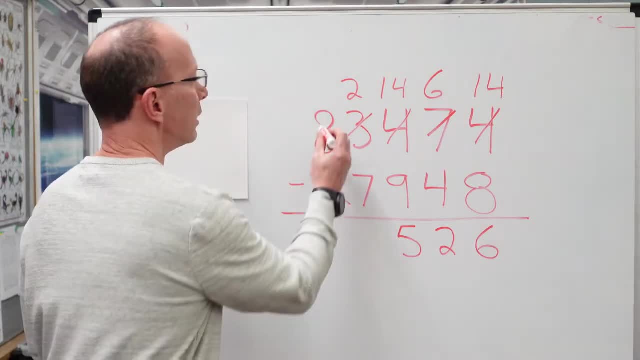 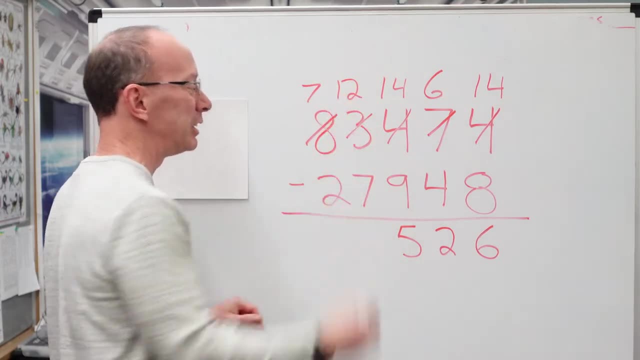 Hey, can I borrow some cookies over there? Sure Crude, Put a line through that eight there, Make that a seven And this becomes a 12.. 12 minus seven, Seven, eight, nine, 10,, 11,, 12.. Here we. 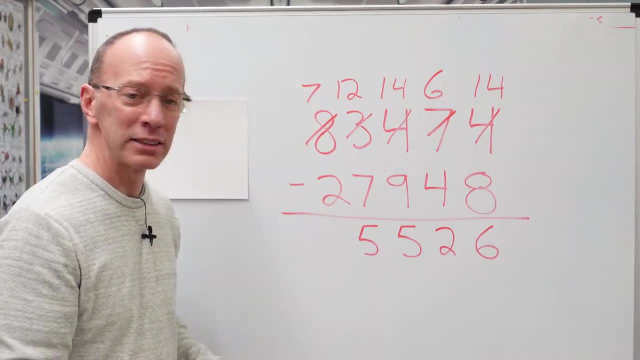 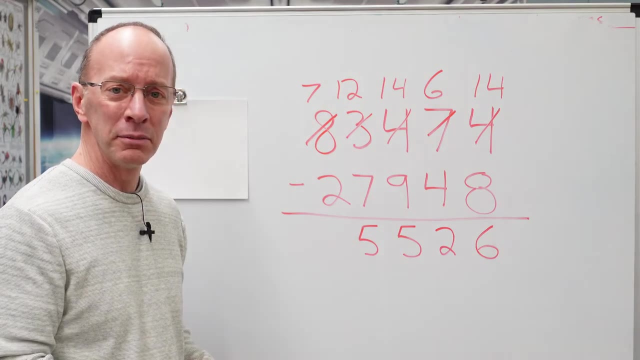 got a five right here. Let's work on our last number. Hey, it wasn't too bad, was it? We just covered these numbers up. It's easy cheesy working this way: Seven minus two. Let me see: Seven minus two, two, three, four, five, six, seven. 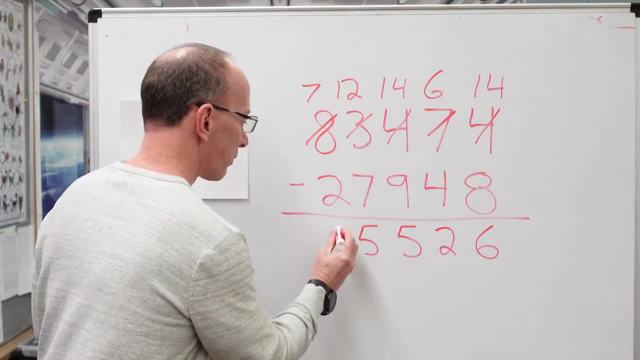 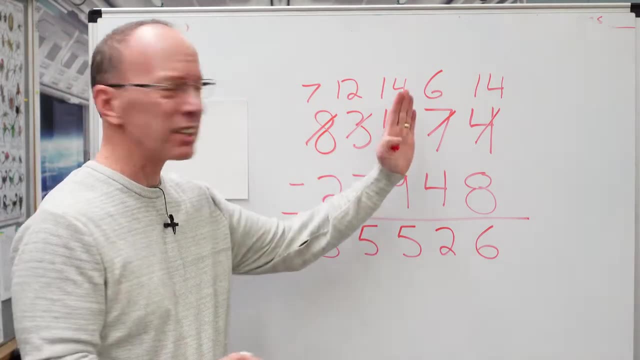 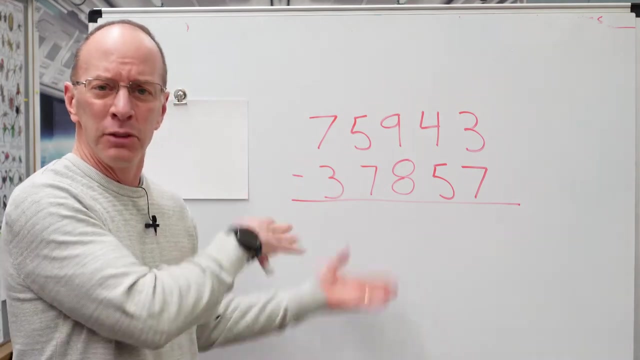 Five, Seven minus two is five. There's our answer. This is a gigantic problem And it was easy to do it. if we just start to cover these numbers up. Hey, would you like to try another number? Let's do it. Yeah, Hey, welcome back. Okay, Hey, if you want to work on this problem with me, you could. 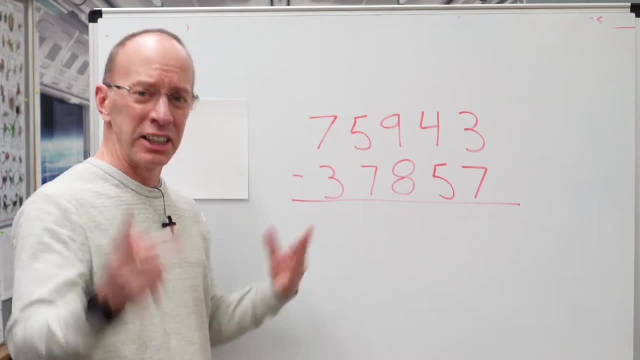 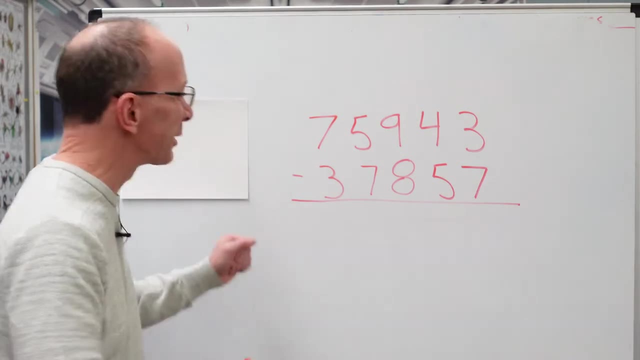 freeze the video right now. copy this problem down and then you can check the answer when we go over it. So right now, go ahead and freeze the video. All right, Welcome back. Okay, Let's start this problem here Once again, don't get nervous, Don't get. 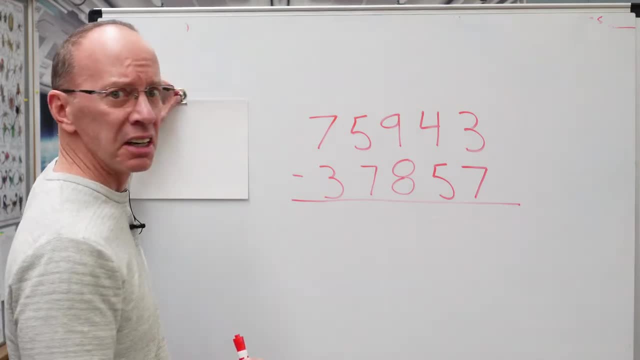 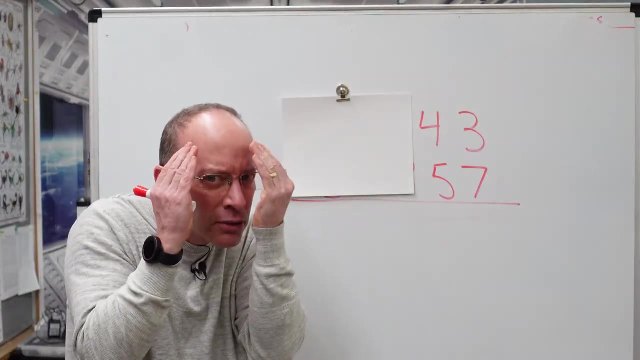 nervous. There's a bunch of numbers right here. All right, Just kind of cover it up right there. It's like sometimes when you see a scary movie, it's like, oh my goodness, And you kind of peek through there a little bit. So don't worry about it, I'm just going to cover most of these numbers. 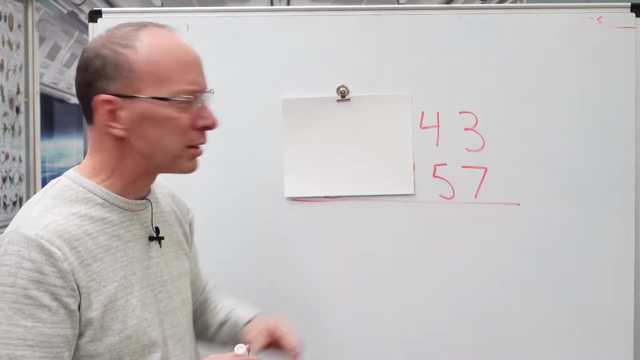 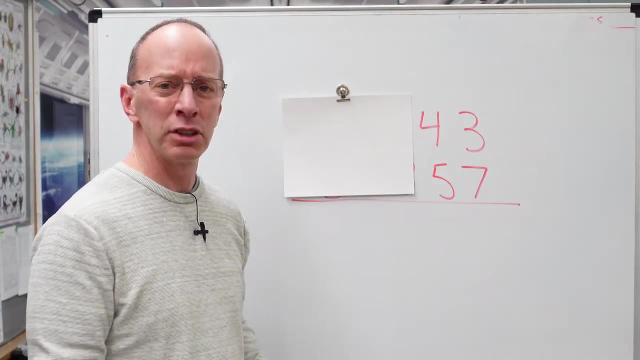 up. I'm going to leave these two right here. I'm not too worried about these, So let's go ahead and subtract these two. Can I do it? I've got three cookies. You want to take seven? No way, No, This number's too small. We need to make it bigger, Bigger, Yeah, So I need to borrow. 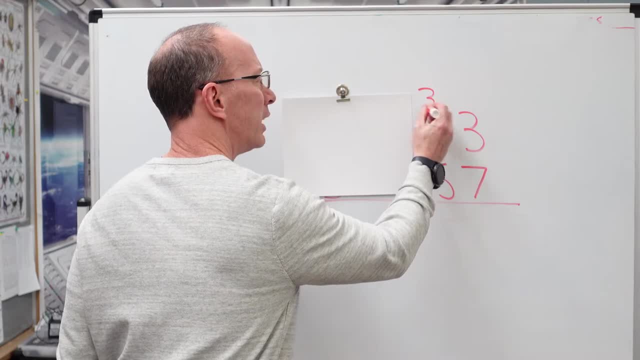 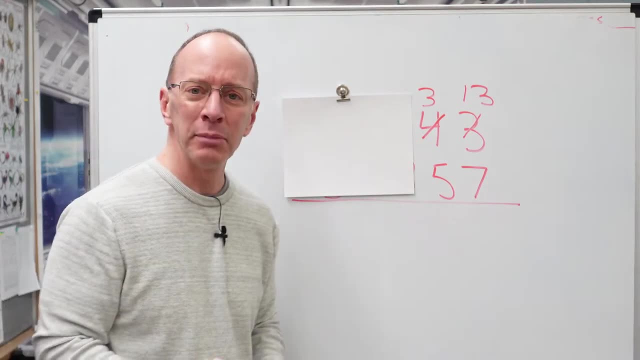 over here. Borrow one from the four, That will be a three. I'm going to add that 10 to the three, That'll be a 13.. My board's kind of wobbling there. All right, 13 minus seven, What is it? 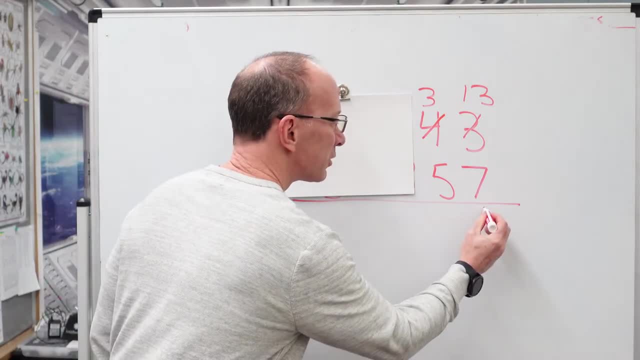 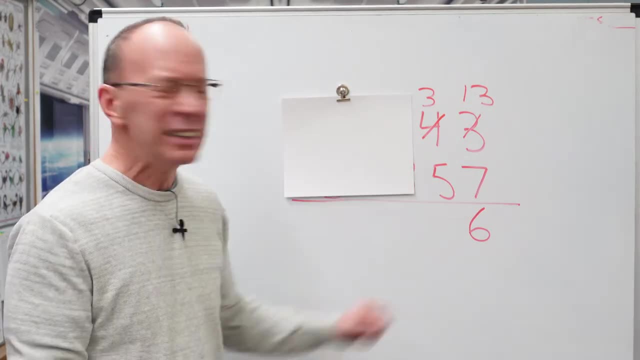 That's right. Six pickup sticks. We'll put a six right here. Now we got a three. Can I take five from there? No, I can't do it Too small. Got to go over to the next door neighbor. I think I can move this paper out here. 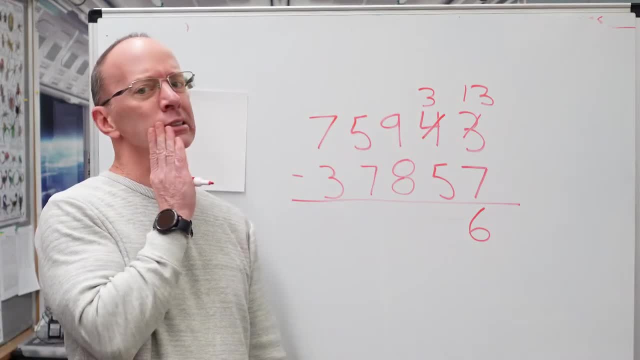 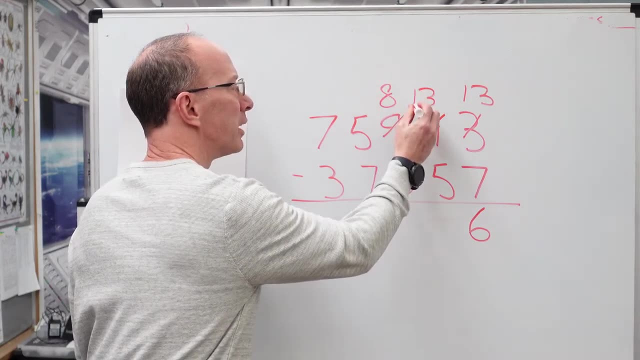 now Need to borrow from the nine. Hey, Mr Nine, could I borrow one from you? Sure, So I cross the nine out, Make that an eight And this will be a 13.. 13 minus five, What is it? What do you think? 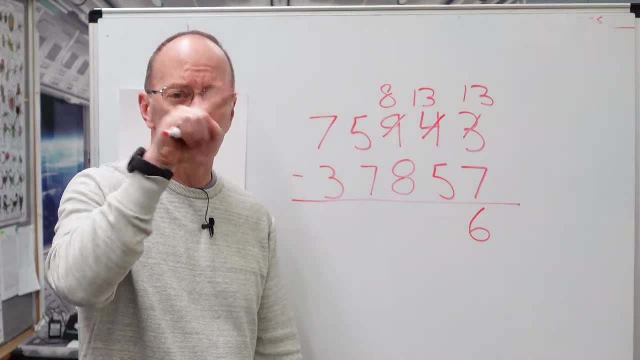 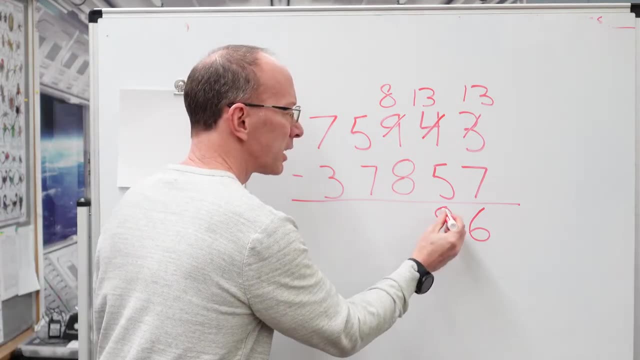 Five, six, seven, eight, nine, 10,, 11,, 12, 13.. That came to be eight. Yeah, Eight, nine, 10,, 11,, 12, 13.. Always want to check, Always want to check. Here's my eight. Can I do this? Eight minus eight Don't. 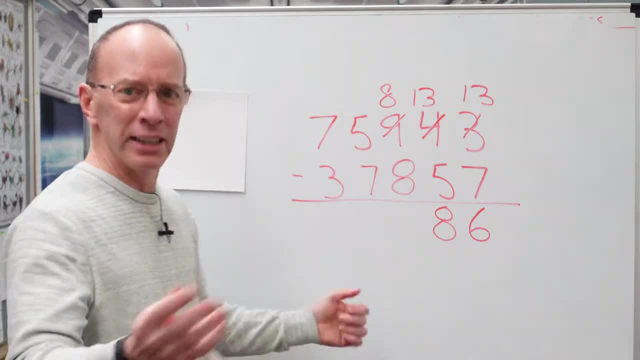 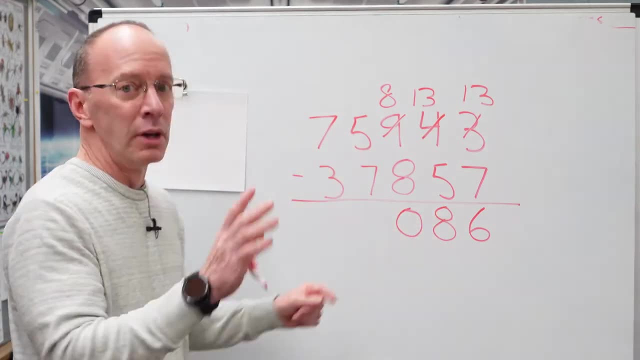 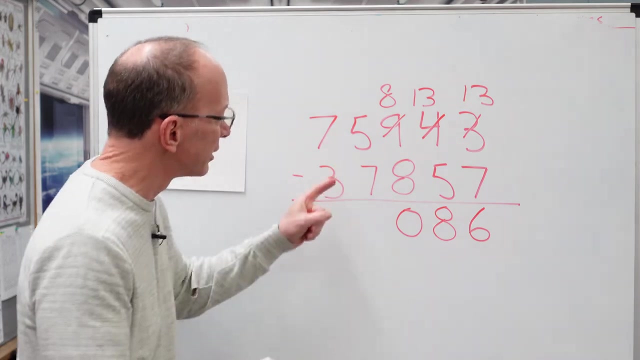 be late. Eight minus eight is zero. That's right, Taking eight away from eight. This is a simple zero. Did not have to borrow it all. All right, If you need to get a glass of lemonade right now, you can do it, because this is a gigantic problem. Okay, Let's go ahead and work on this. Can't do. 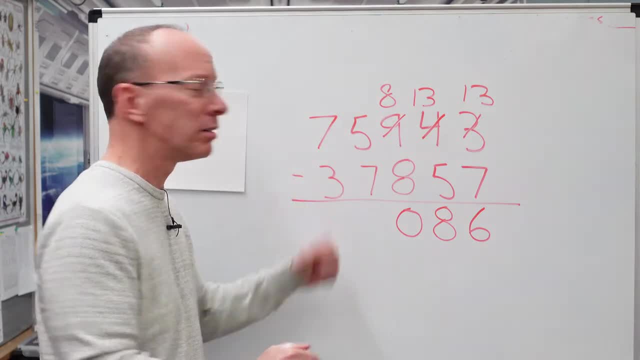 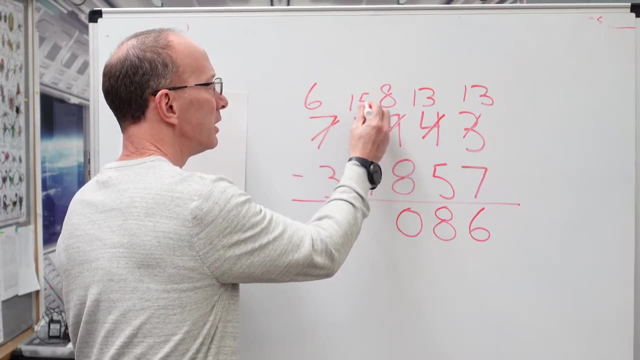 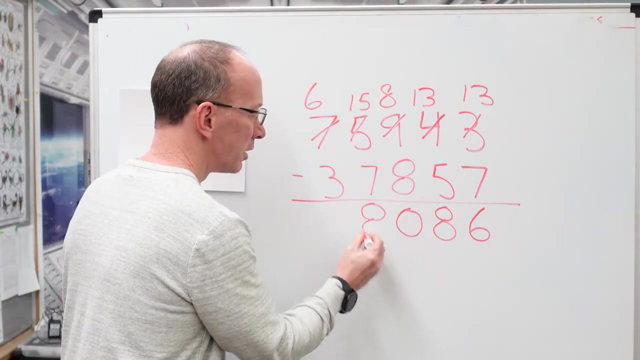 it, can we? We noticed that this number right here is too small. Need to borrow. Thank you, Mr Number seven. Got to borrow one from you And I make this a 15.. 15 minus seven. Yeah, eight, That's right. Hello, Mr Eight, He's always late. Get it Eight late. 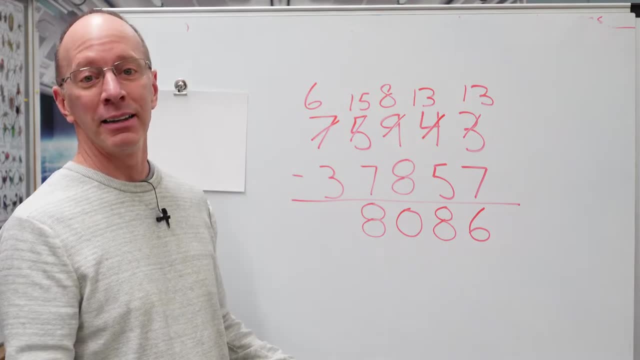 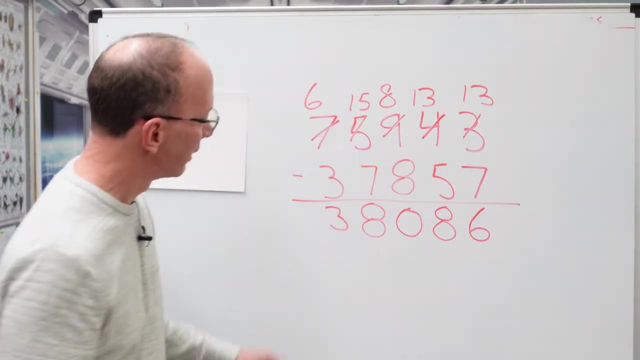 All right, Six, Six minus three. That one is so easy. You can finally take a breather. We can do that Three. There's our gigantic answer to this problem. Hey, you ready to do one more? I got a little. 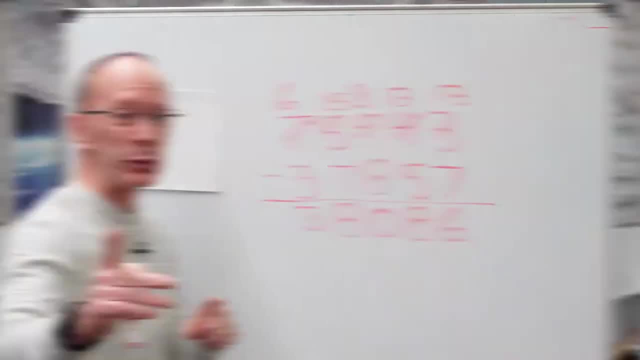 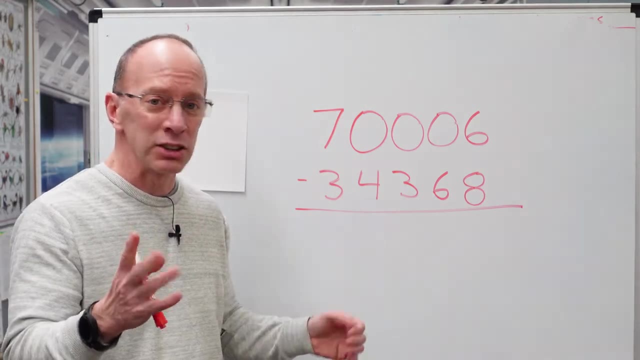 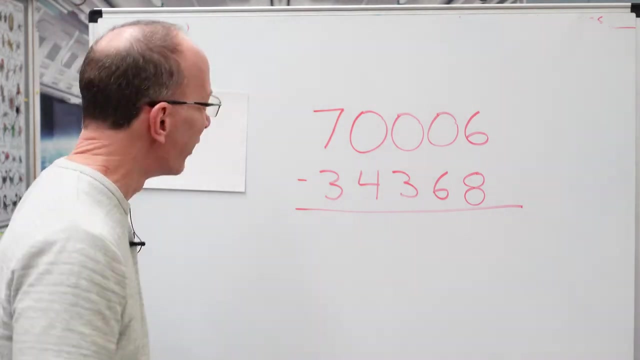 tricky one for you. All right, Let's do it. All right, Welcome back. Hey, like I said, if you want to freeze the video right now, do this and then we'll recheck it. So go ahead and freeze the video. All right, Welcome back. Okay, Whoa, Hey, did you notice something right here? 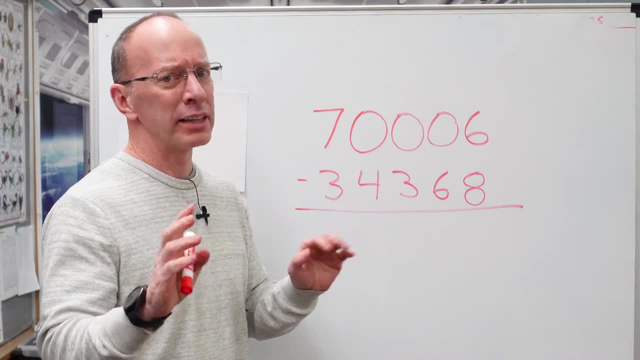 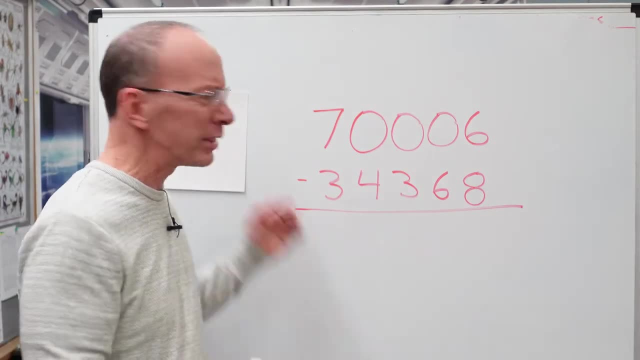 We got a lot of zeros. Don't get nervous about that. Don't get nervous. We could. you know what? I think? I think I'm getting confidence. I think I I think we can do this without this piece of paper, right there. All right, let's do it. Let's start. 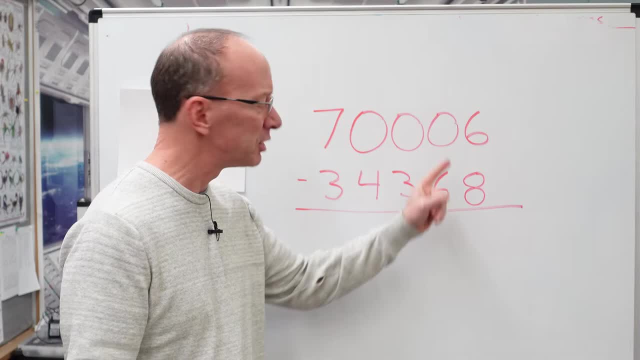 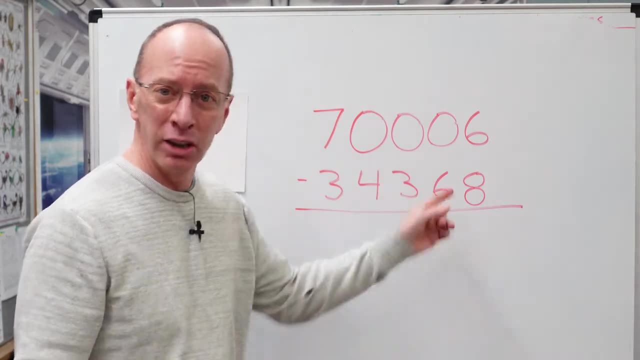 with the ones Here. we notice that this number is too small. You always want that number over here, kind of big like a big old hat to cover yourself from the rain I need to borrow. So you go over to the next door neighbor. Whoa, You notice that next door neighbor. he doesn't have any cookies. 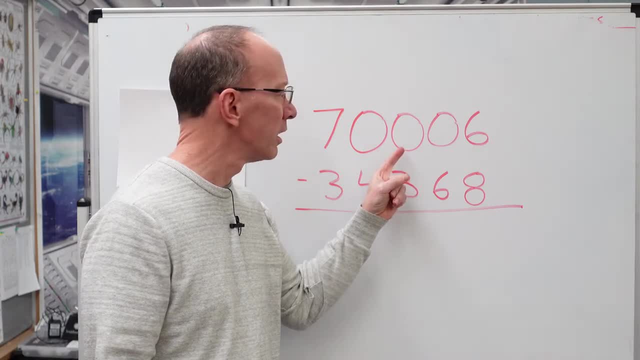 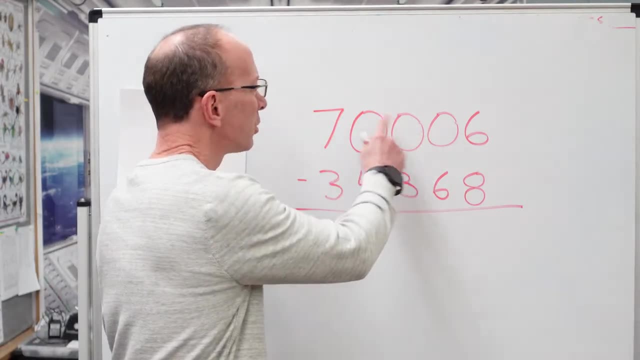 Let's go next door. Whoa, No more cookies over here. No more cookies. What's the deal? Everybody is out of cookies. We got to go one, two, three, four houses down to get some cookies over here. So all right, At least. 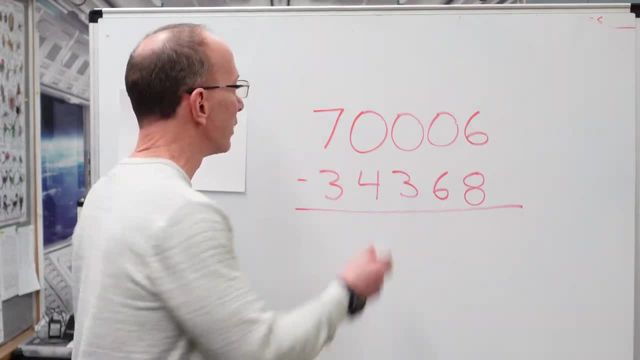 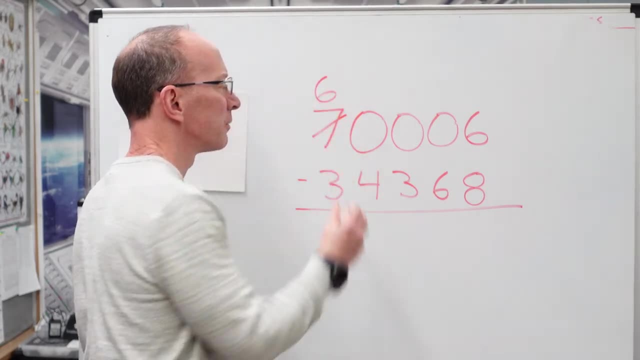 we got some cookies over here, So we need to borrow one from the seven. I'm going to show you a little trick on how to do this. I take one from the seven, and this will be a six. Now, what I usually would do: 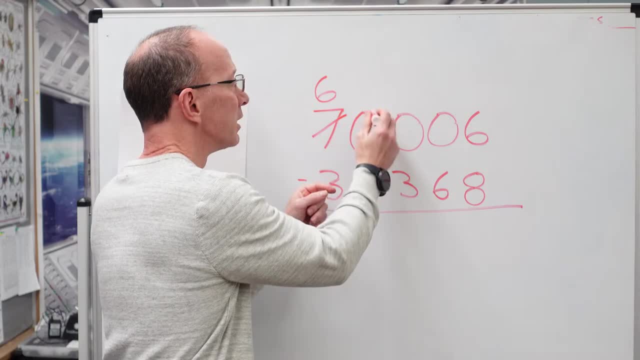 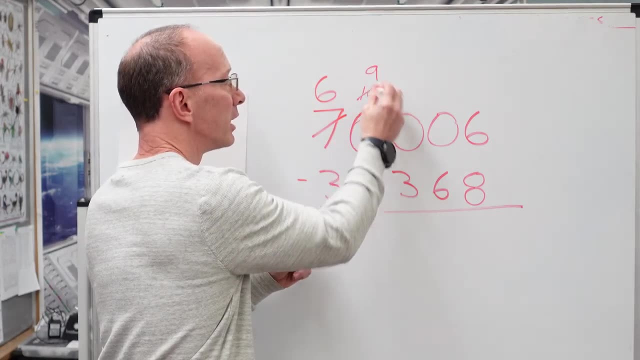 is start from here. I'd cross this out, and this would be a 10.. All right, But then I would have to borrow one from here, And so I'd have to cross that out, and that would have to be a nine. And 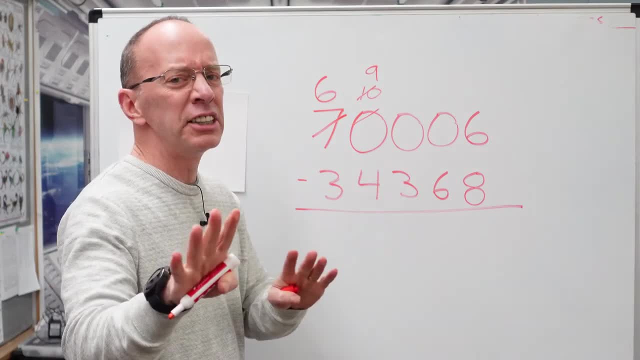 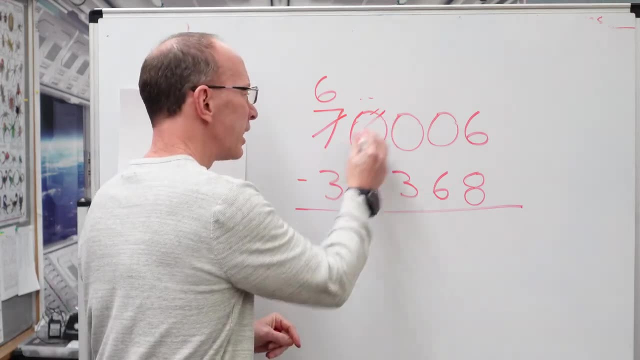 then this would be a 10 and it gets. there's an easier way to do it. You just let's take it easy. You know you're going to have to turn that into a nine, So just put a line through there. 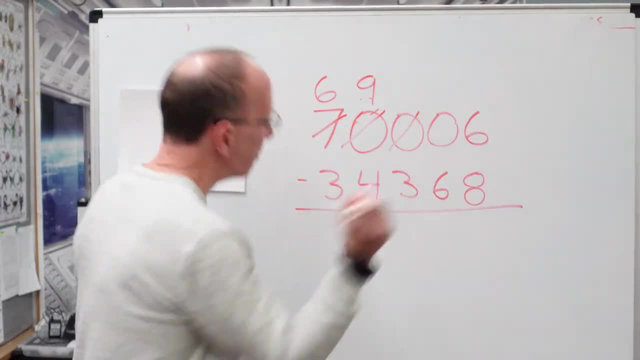 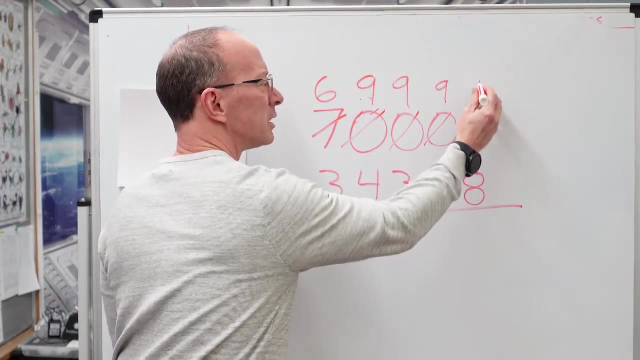 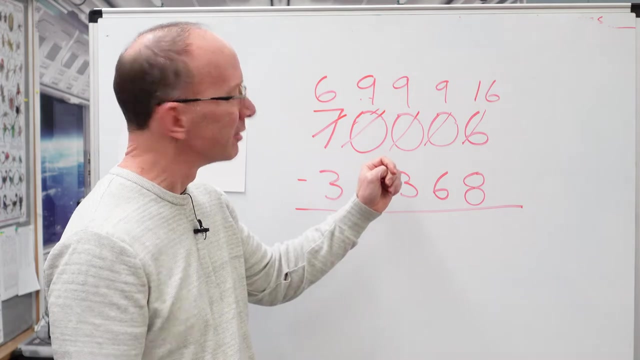 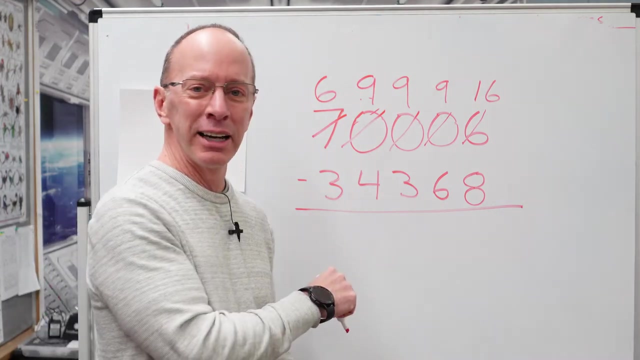 make it a nine, put a line through there. make it a nine, put a line through there, make it a nine, And this one becomes 16.. Can you see that? Pretty easy, isn't it? All right? So now we go ahead and subtract 16 minus eight. Don't be late, Come on, You can do it. 16 minus. 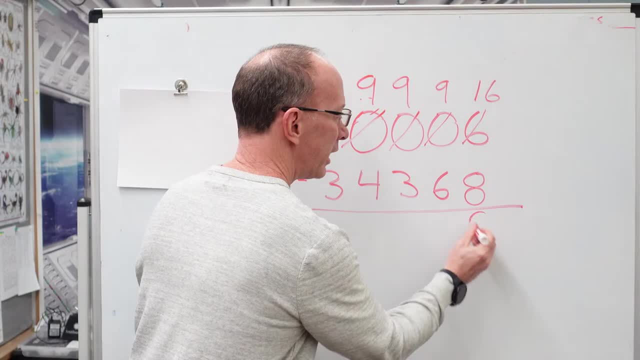 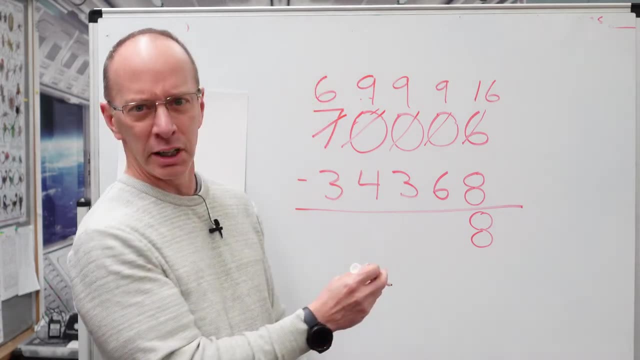 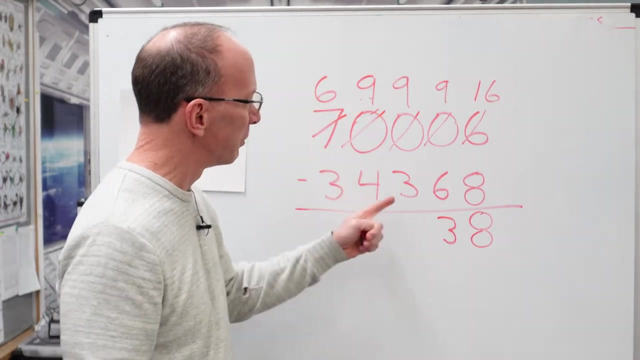 eight. double fact eight. Put the eight right here. Nine minus six, six, seven, eight, nine, three- I think I'm singing because I'm happy as I'm almost done These math problems- And then you can get going on with the rest of your day. Nine minus three. 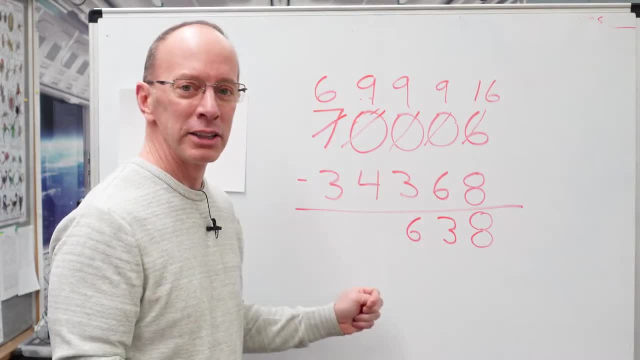 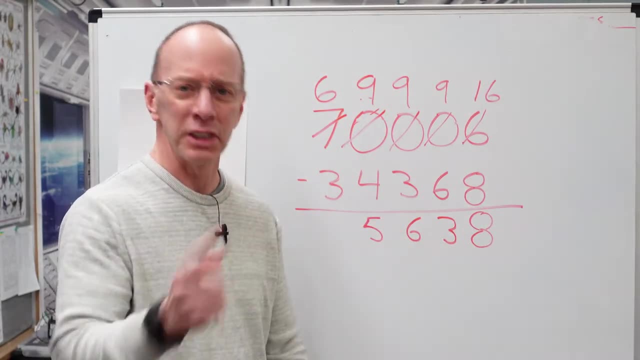 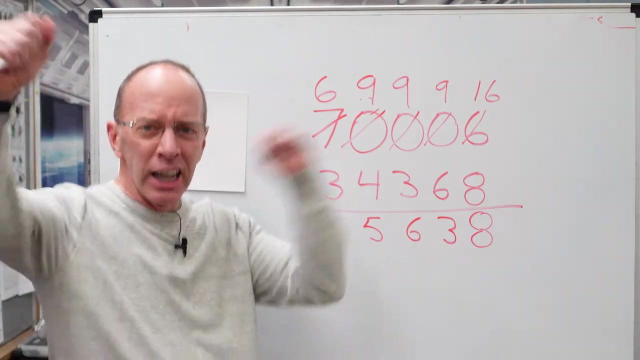 six, nine minus four, five, cinco, cinco, Uno, dos, tres, cuatro, cinco, Muy bien, Muy bien. Last number, Last number, Can we do it Six minus three? Yes, Three, Tres, We did it High five. 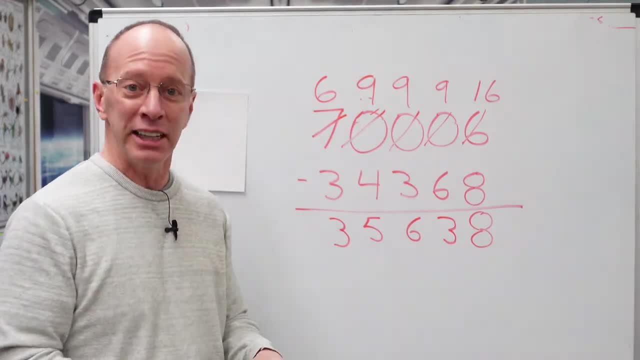 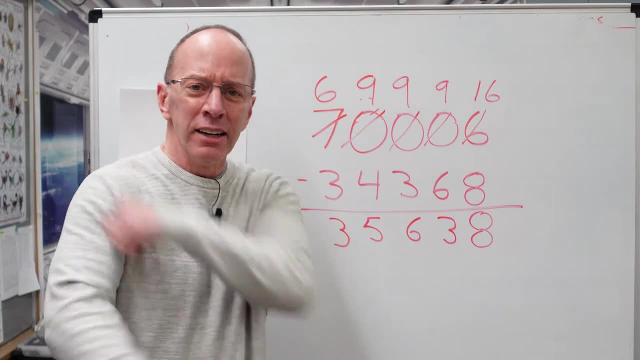 I don't know if you can High five on the video there, but hey, you did it, You graduated. Hey, I hope you had a great day today. Make sure you check out my other videos on here And, like always, have a fun day, Adios. 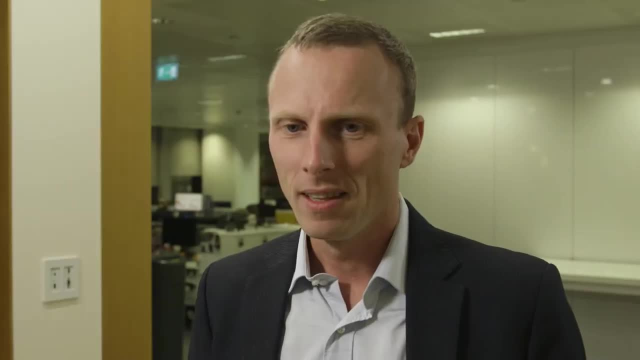 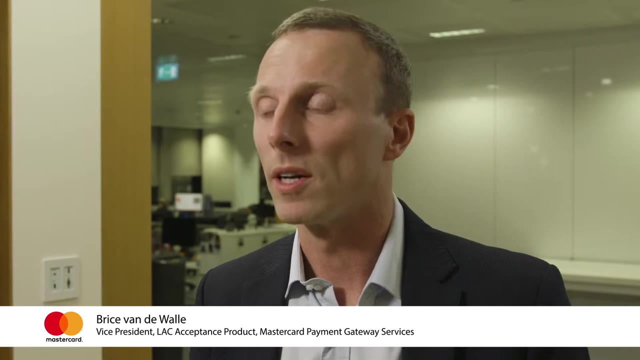 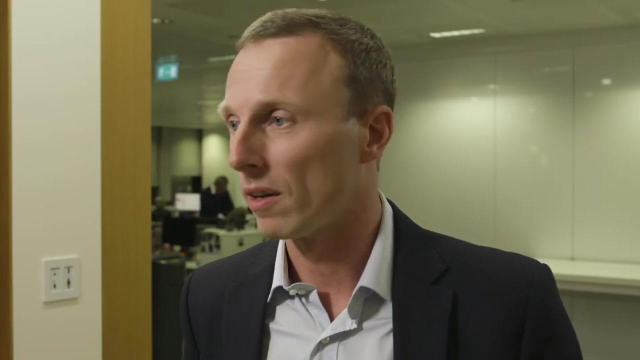 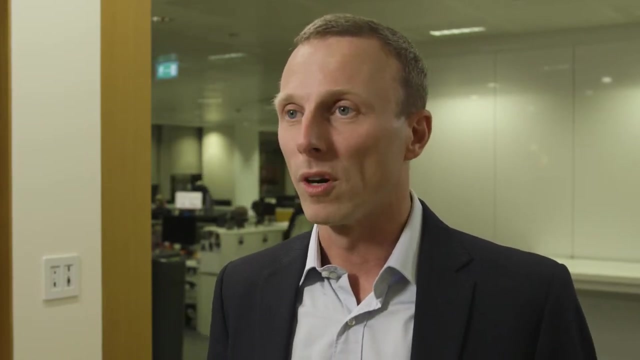 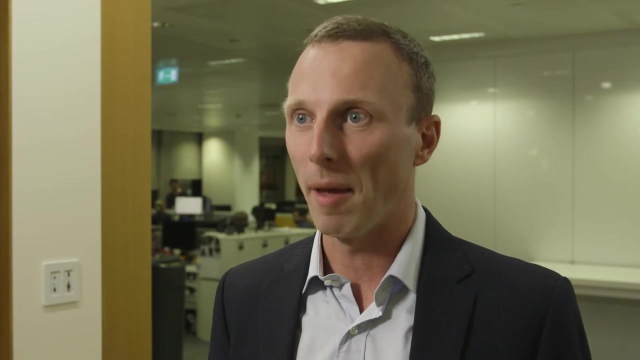 Things are becoming increasingly complex in order to follow your customer right. People are increasingly knowledgeable how to use their mobile, their tablet, their PC or shop in store right. So you want to have a solution that can basically support your customers to pay wherever they want, whenever and however they want. So I think MPGIS is again bringing 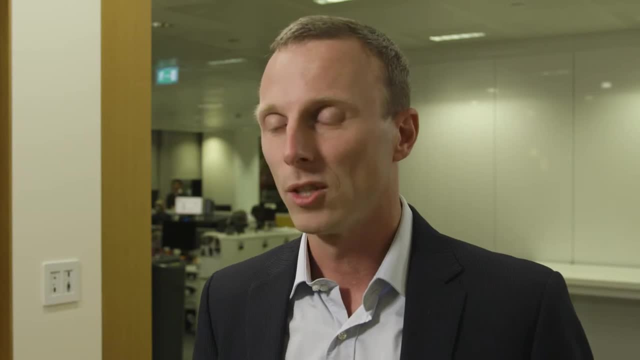 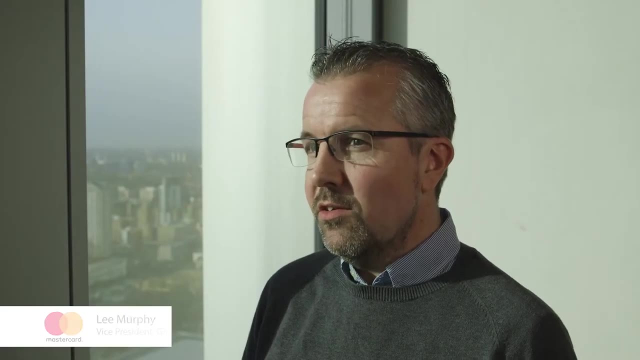 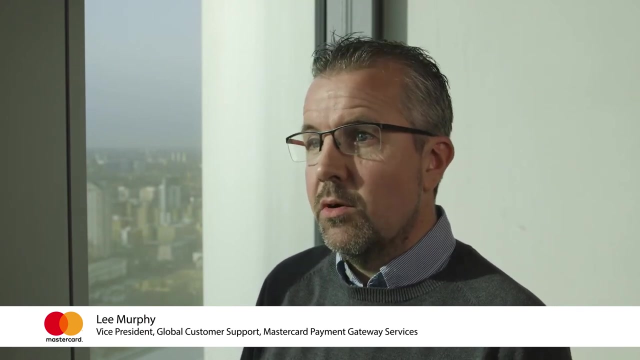 that kind of flexibility with an omnichannel solution, so you don't really need to worry anymore about what is your customer needs. The top tip for merchants is to understand their customer, Understand the friction points that their customers go through, and to be able to respond to them and use Mastercard.